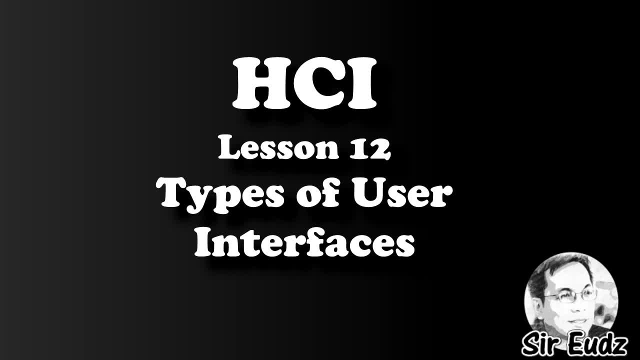 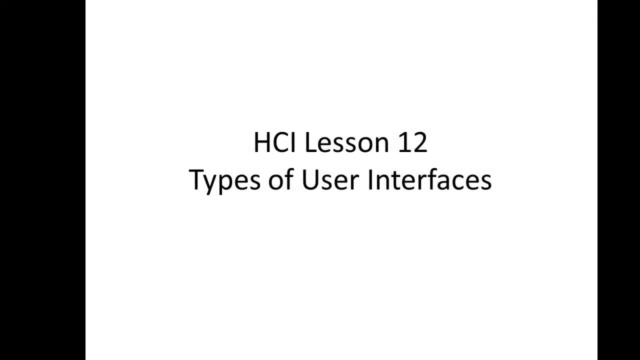 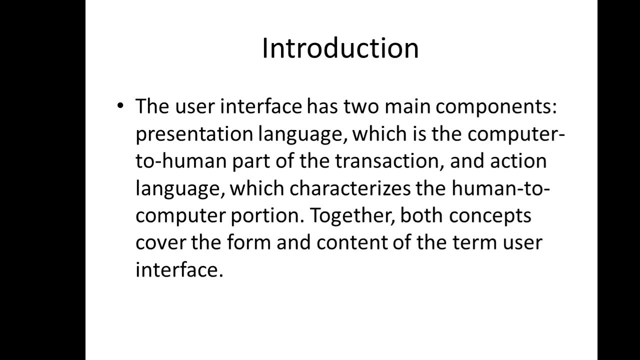 HCI, Lesson 12. Types of User Interfaces. So this is the 12th of the series of video lectures for HCI Introduction. The user interface has two main components: The presentation language, which is the computer-to-human part of the transaction, and an action language. 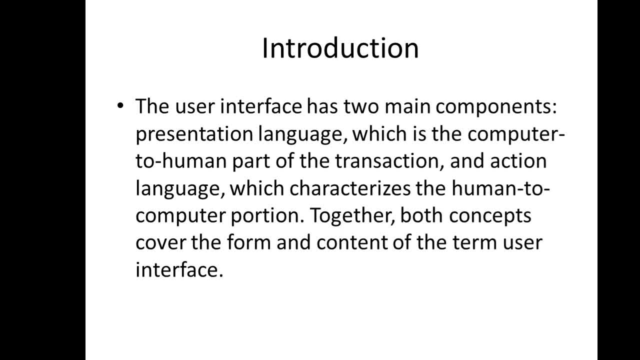 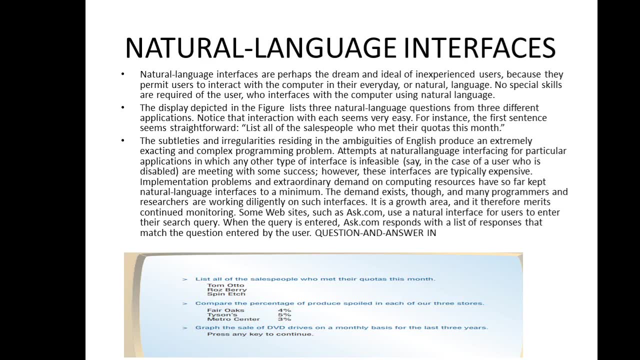 which characterizes the human-to-computer portion. Together, both concepts cover the form and content to the term user interface, The natural language interfaces. Natural language interfaces are perhaps the dream and ideal of an expert, Experienced users, Because they permit users to interact with the computer in their everyday. 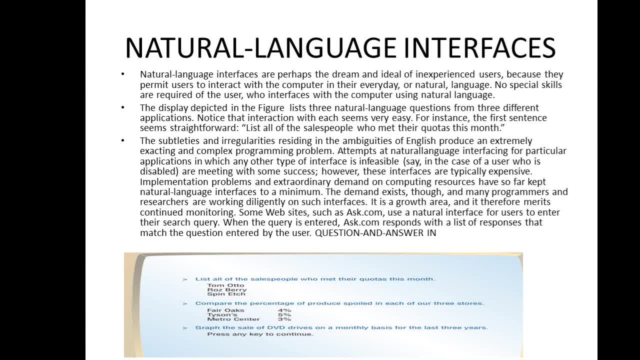 or natural language. No special skills are required of the user who interfaces with the computer using natural language. The display depicted in the figure, so that's below, lists three natural language questions from three different applications. Notice that the interaction with each of the three languages is a natural language. The interaction with each of 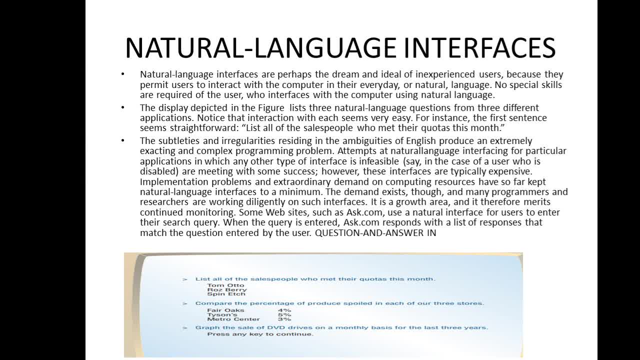 the three languages seems very easy. For instance, the first sentence- seems straightforward- Lists all the salespeople who met their quotas this month. So the subtleties of an irregularity residing in the ambiguities of English produce an extremely extracting and complex programming. 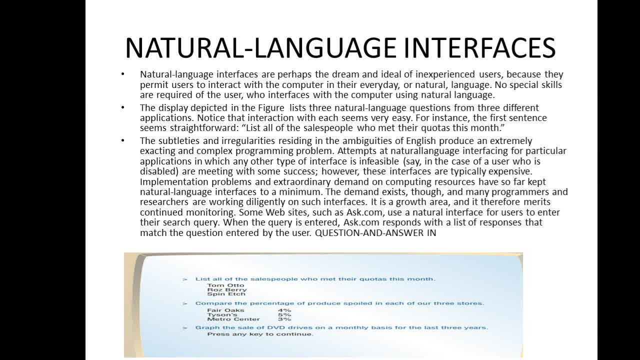 problem. Attempts at natural language interfacing for a particular application in which any other type of interfaces is invisible, Say in the case of a user Who is disabled, Are meeting with some success. However, these interfaces are typically expensive. Implementation problems and extraordinary demand on computing resources have so far kept natural. 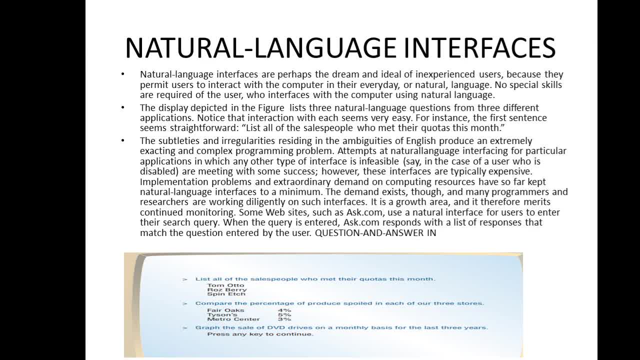 language interfaces to a minimum. The demand exists, though, and many programmers and researchers are working diligently on such interfaces. The demand exists, though, and many programmers and researchers are working diligently on such interfaces. The demand exists, though, and many programmers and researchers are working diligently on such interfaces. 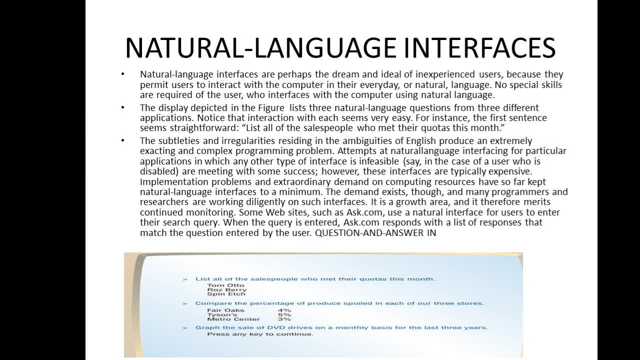 It is a growth area and it therefore merits continued monitoring. Some websites, such as Askcom, use a natural language for users to enter their search query. When the query is entered, Askcom responds with a list of responses that matches the question entered by the user. 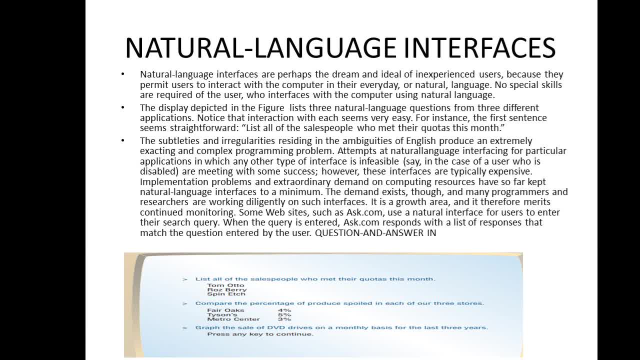 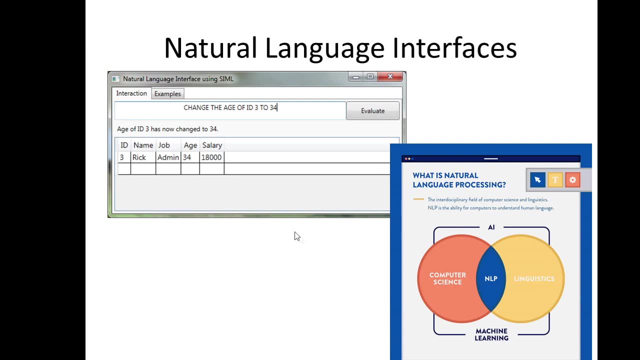 So question and answer interface. So actually google, the google search engine, also some sort of make use of natural language. so here are even some examples of natural language. so here we can see here that the user just typed: change the age of id3 to 34, which is very straightforward. 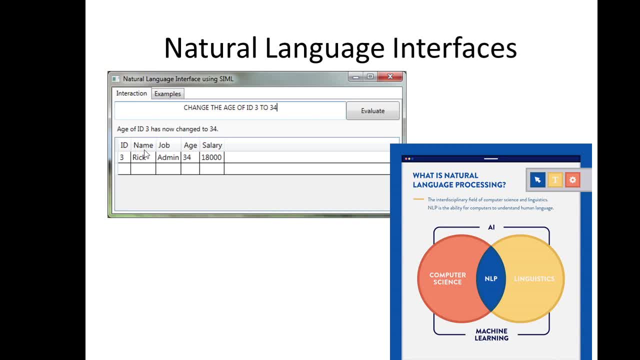 so this will change the id, the age of this record with an id3, to 34.. so, unlike if you use the real select statement, where you're going to use, where you're going to follow a particular syntax like update, a update, whatever, the name of the stable is then set: h equals 34 where id equals. 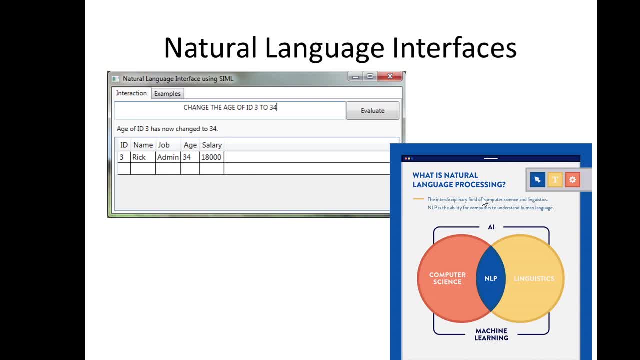 three, that's sql. so what is natural language? if we're going to look at this at a glance, natural language is actually a combination of computer science and linguistics. so we have to combine them to arrive at our natural language processing, and of course it requires ai and machine learning. 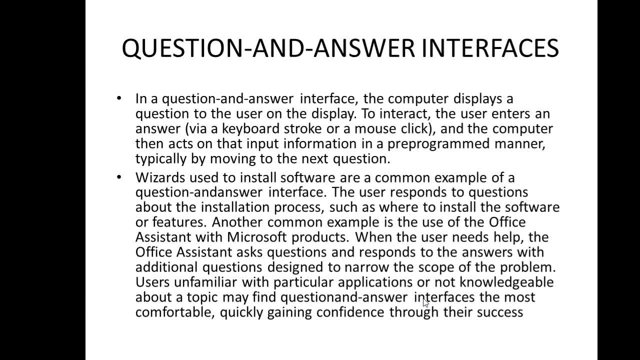 then we have the question and answer interfaces. in a question and answer interface the computer displays a question to the user. on the display to interact, the user enters an answer, maybe by a keyboard stroke or a mouse click, and the computer then acts on that input information in a pre-programmed manner, typically by moving to the next question. 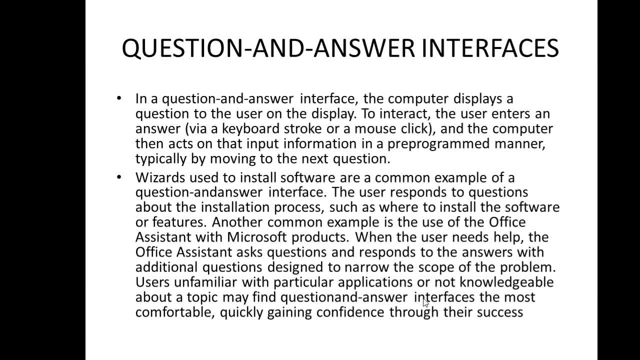 wizards used to install software are a common example of the question and answer interface. the user responds to the questions about the installation process, such as where to install the software or features. another common example is the use of the office assistant with microsoft products. when the user needs help, the office assistant ask questions and 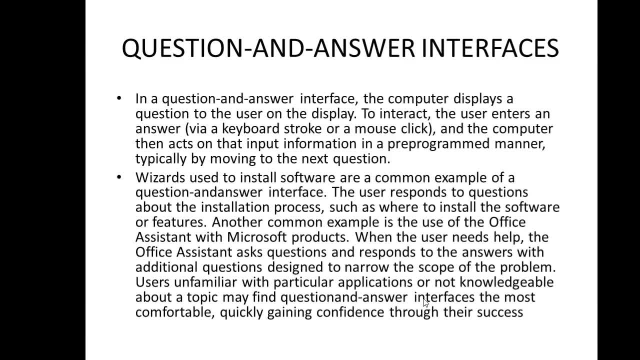 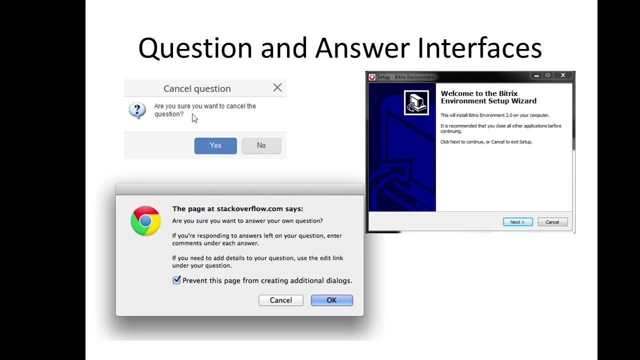 responds to the answer with additional questions designed to narrow the scope of the problem. users and familiar with particular applications or not knowledgeable about the topic may find question and answer interfaces the most comfortable and quickly gaining confidence through their success. so here are examples of question and answer interfaces. so say, are you sure you? 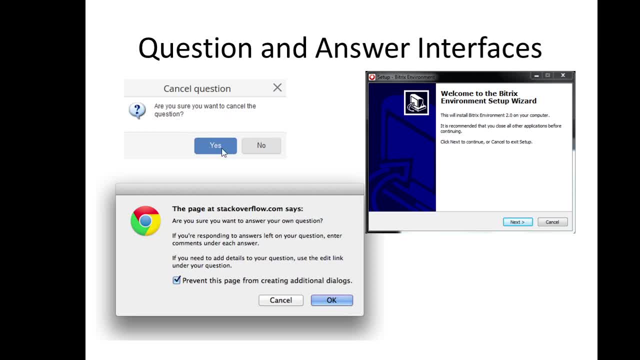 want to cancel the question. so that's already the question. so, yes or no? then here we have another here dialog. so the the page that stock overflow says: are you sure you want to answer your own question? if you're responding to answer blah, blah, blah, so we can click ok or maybe cancel. 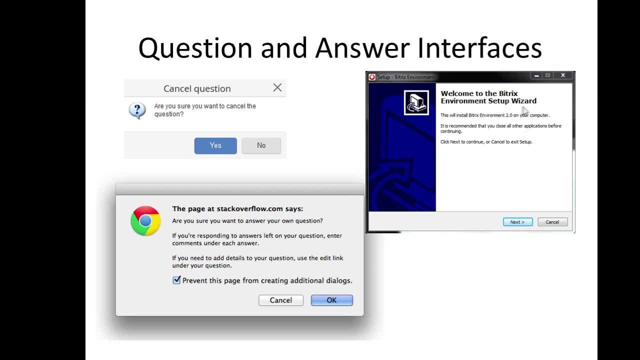 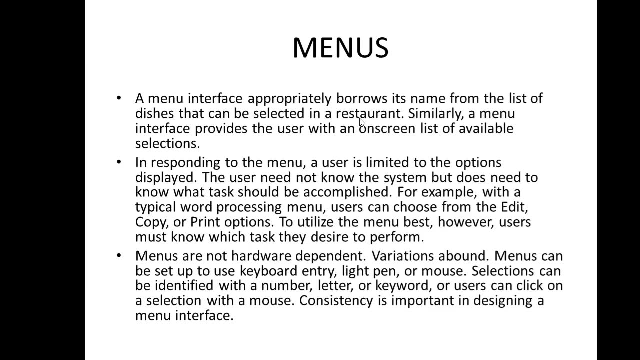 and here's another one: welcome to bittrex. environment setup so, and then you can click next or maybe cancel. so these are examples of question and answer interfaces- menus: a menu interface appropriately borrows its name from the list of dishes that can be selected in a restaurant. similarly, a menu interface provides the user with an on-screen. 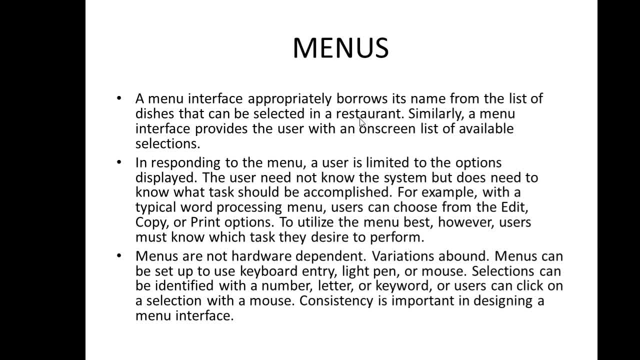 list of available selections. in responding to the menu, a user is limited to the options displayed. the user need to know the system, but does not does need to know what tasks should be accomplished, for example, with a typical word processing menu. users can choose from the edit, copy or print options. 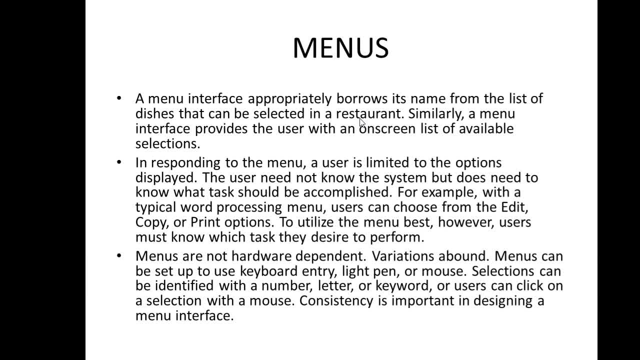 to utilize the menu best, however, users must know which tasks they desire to perform. menus are not hardware dependent. variations are bound and menus can be set up to use keyboard entry like pen or mouse. selections can be identified with the number, letter or keyword, or users can click on the selection with the mouse. 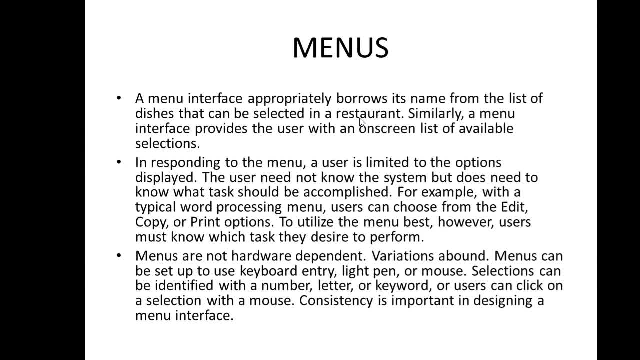 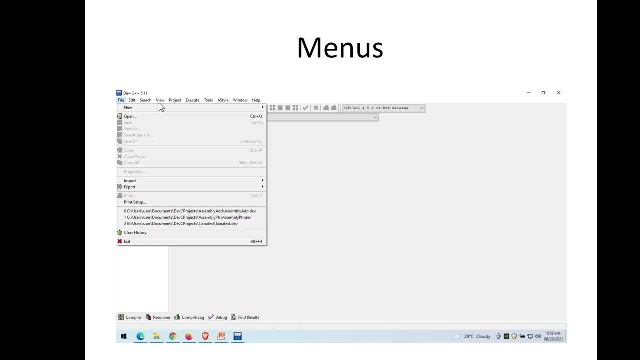 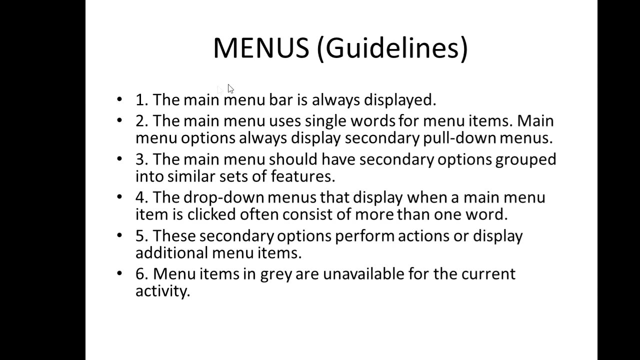 consistency is important in designing a menu interface. so here is an example of an application using a menu interface. so this is actually devc. so these are menu. so we have read the main menu and we have created the secondary options. so menu guidelines now. so to decide menu. so the main menu bar is always displayed. so that should be. 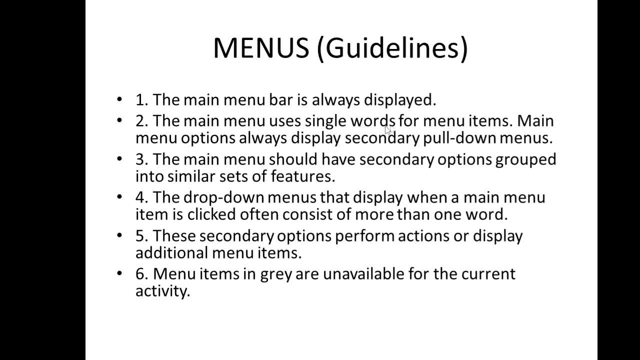 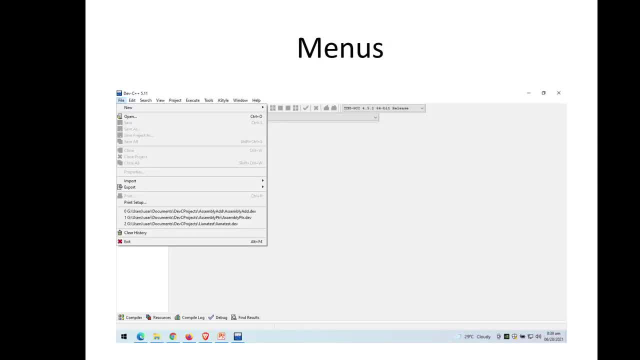 our first guideline. the main menu uses single words for menu items. so main menu options always display secondary pull down menu. so if you got to look at this, this is our main menu and you notice that it is only using single word. and these are now our secondary options. 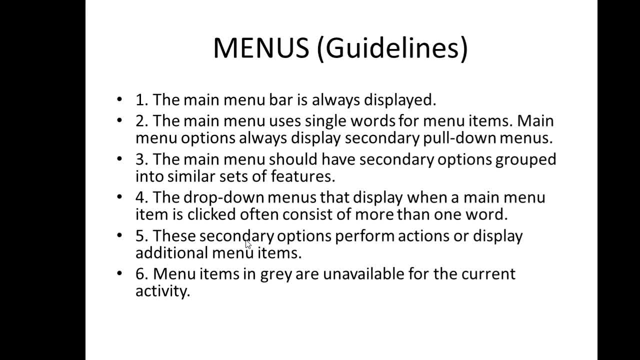 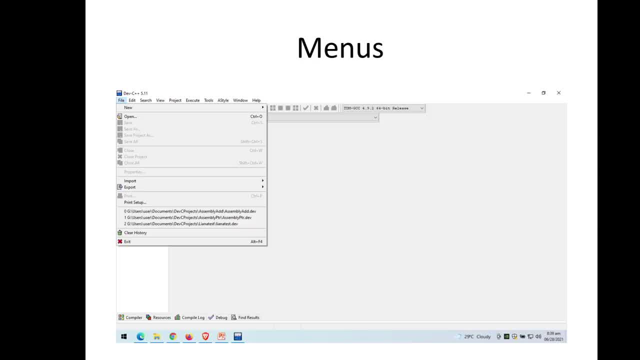 then the third one. the main menu should have secondary options grouped into similar sets of features. so again, this is our secondary menu. you notice it is also grouped, the features. so this is for opening and saving, this is for closing the project, this is for import and export, so it is grouped. 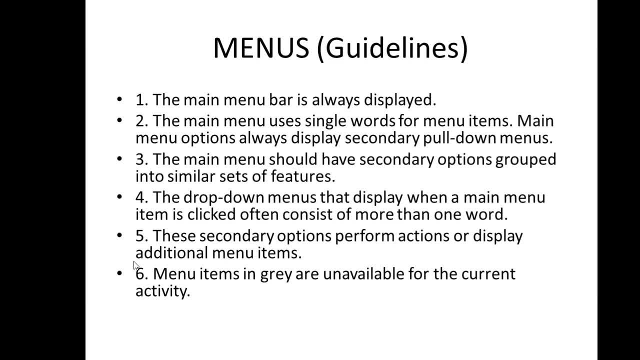 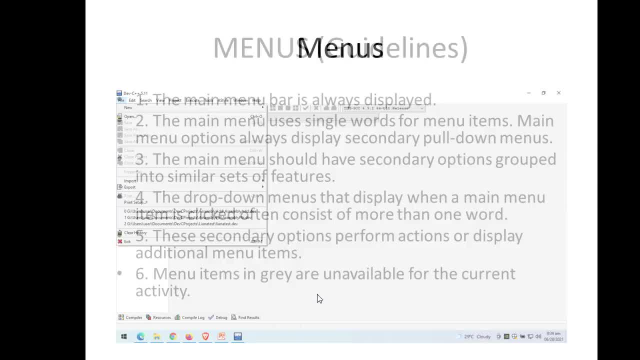 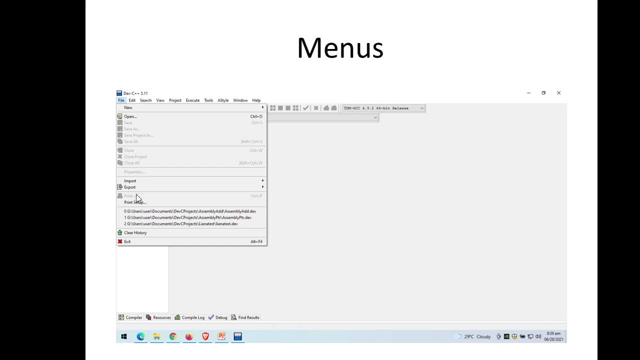 the drop down menus that display- when i mean main menu items, click often consists of one or consists of more than one word. so if you're going to going back at this, so some here are more than one word. so print setup. so we have here: close project, save project, save us. so these are examples of menu. 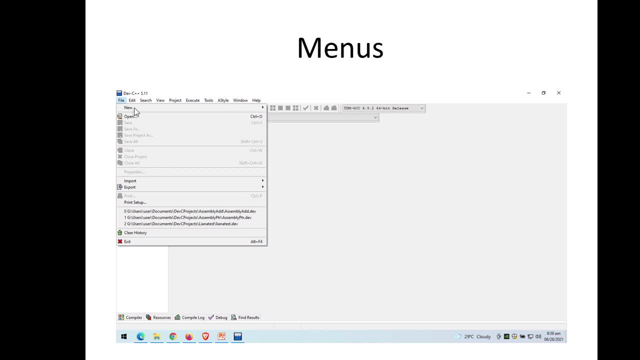 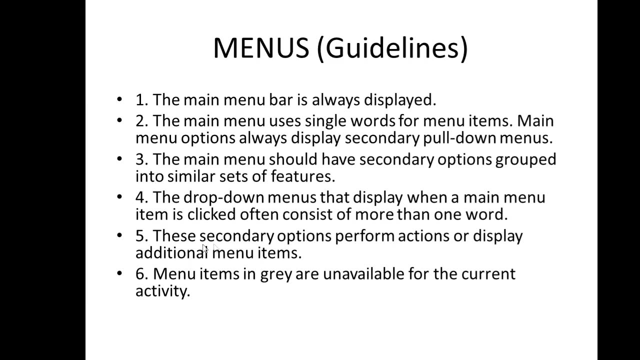 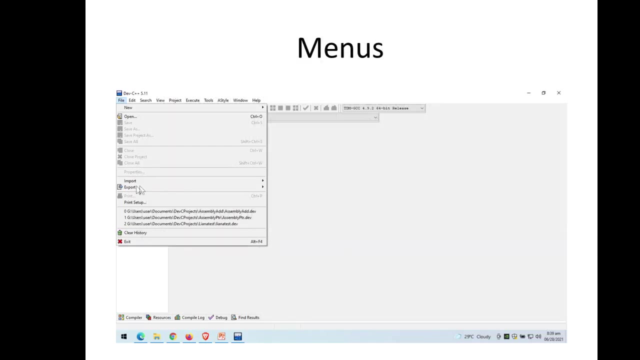 so, unlike the main menu, which should be single word, the secondary one can be more than one word. then this secondary options perform actions or display additional menu items. so if you go to look at this, so if you click on this, that's why we have your arrow. 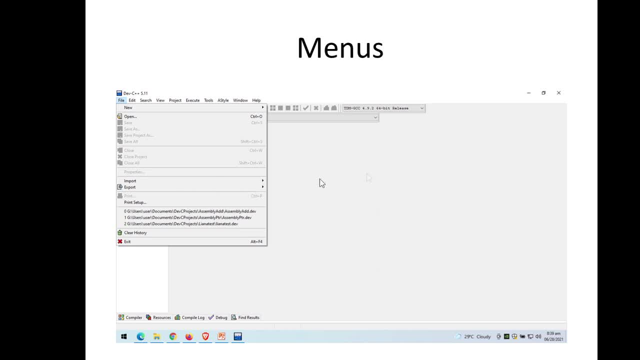 here. that means if you click on this, it will display another set of new, or if you click on open, then this most probably will open a dialog, open dialog box, so it will be performing an action, or it will be opening another menu, just like in this case, in new and so here. so these are indicators. 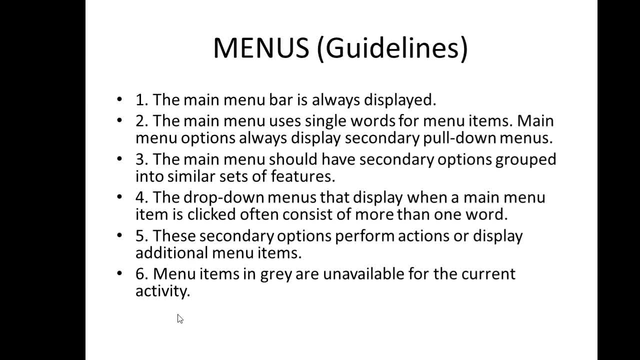 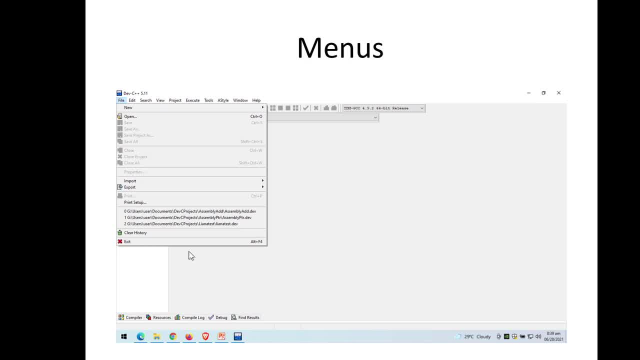 so if you notice that we have a menu item here in gray, so we can see here another menu item. so if you notice there, we have here options that are grade, so that means these are unavailable. so if you notice that we have here options that are grade, so that means these are unavailable. 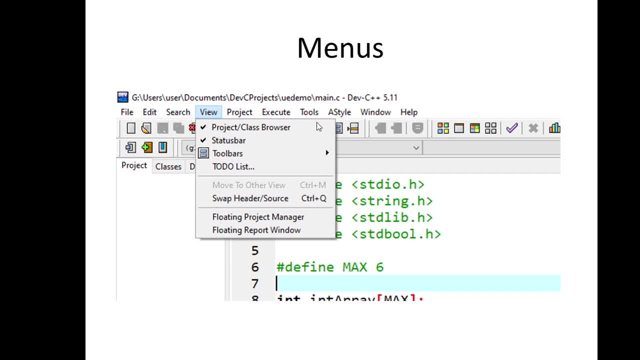 so these are some of the menu guidelines. so here's another example menu. so again, single word. then here we have read our drop down. then this will open another menu because of this arrow here and the words can be consistent, like this thing of more than one word, one word or more, and the grade is actually disabled. 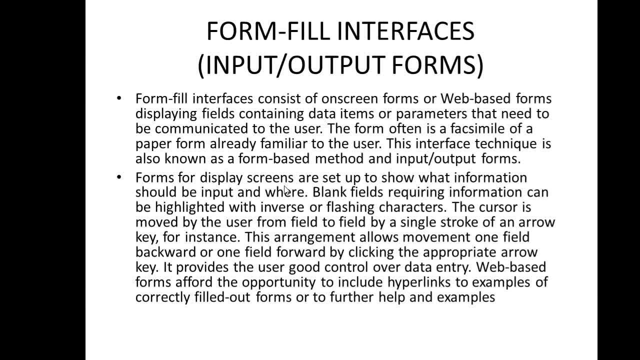 form field interfaces or input-output forms. form field interfaces consists of on-screen forms or web-based forms displaying field containing data, items or parameters that need to be communicated to the user. the form often is a proximity of a paper form already familiar to the user. this interface 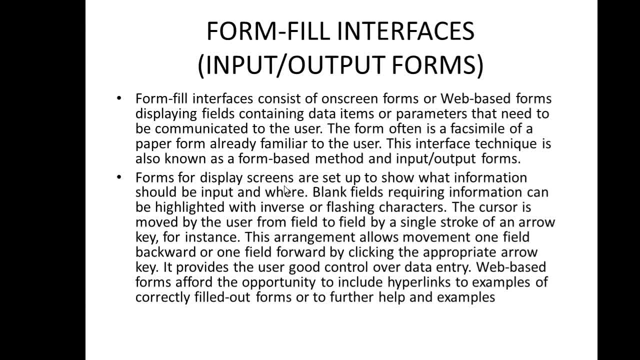 technique is also known as a form based method and input output forms. forms for display screens are set up to show what information should be input and where blank fields requiring information can be highlighted with inverse or flashing characters. the cursor is moved by the user from field to another field to display here. you may notice there. 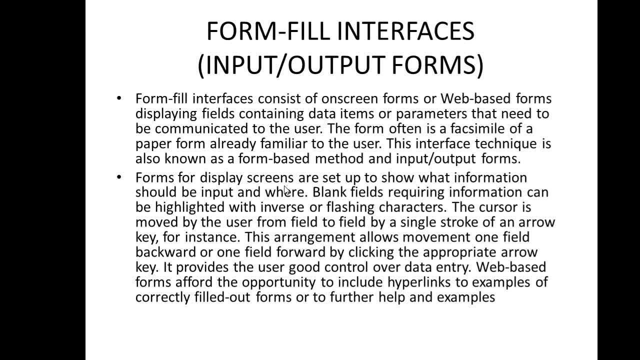 some selected items or labels that the user chose, or things closer to each other to field by a single stroke of an arrow key. for instance, This arrangement allows movement one field backward or one field forward by clicking the appropriate arrow key. It provides the user good control over data entry. 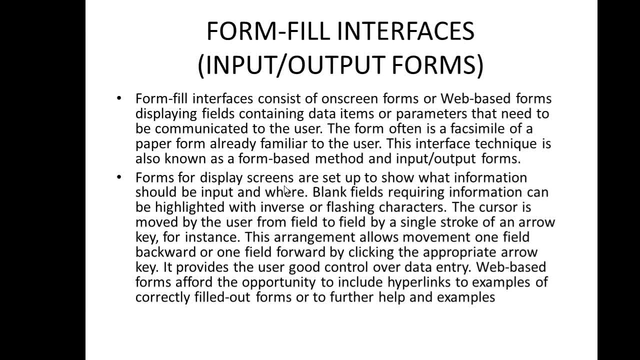 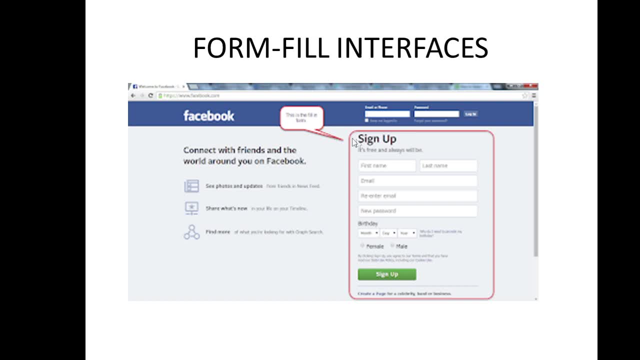 Web-based forms affords the opportunity to include hyperlinks to examples of correctly filled out forms or to further help in examples. So here's an example of a form field interface. So where we can sign up, we have here text boxes and we have here drop-down. 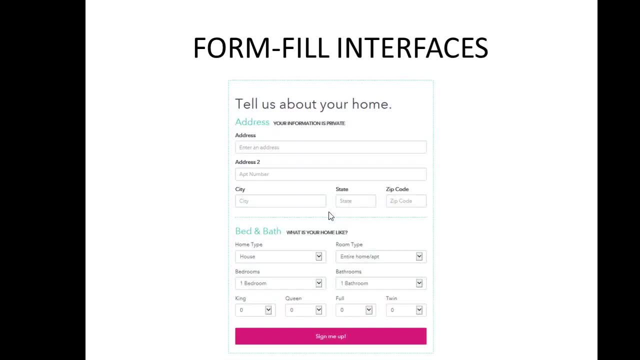 Then we have here a button. Here's another example of a form field interface. So we have here the labels, we have the text boxes, we have drop-down combo boxes And again we have here a button, So form input for displays can be simplified. 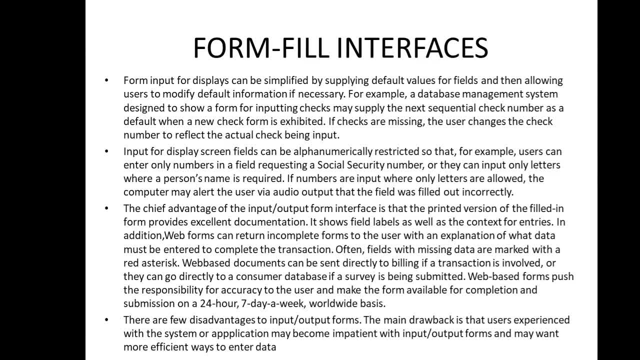 by supplying default values for fields and then allowing users to modify default information if necessary. For example, a database management system designed to show a form for inputting checks may supply the next sequential check number as a default when a new check form is exhibited. 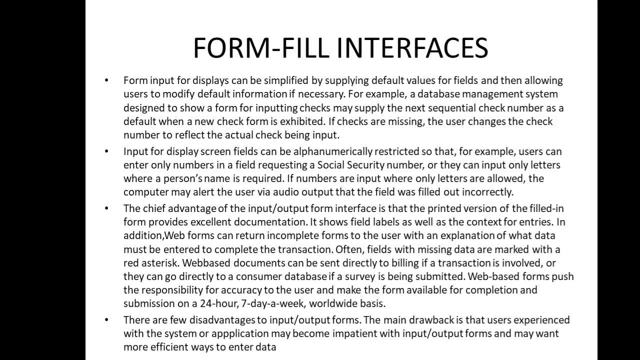 If checks are missed, the user changes the check number to reflect the actual check being input. Input for display screen. fields can be alphanumerically restricted so that, for example, users can enter only numbers in field requesting a social security number, Or they can input only letters where a person's name is required. 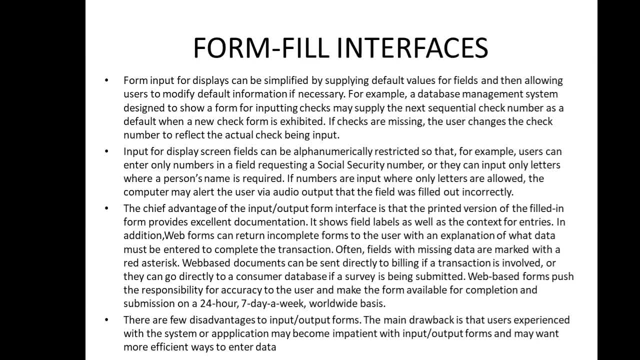 If numbers are input where only letters are allowed, the computer may alert the user. If numbers are input where only letters are allowed, the computer may alert the user. If numbers are input where only letters are allowed, the computer may alert the user. 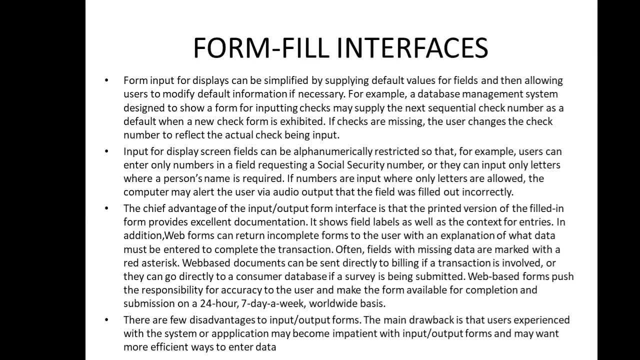 If numbers are input where only letters are allowed, the computer will alert the user. If numbers are input where only letters are allowed, the computer may alert the user. The chief advantage of the input-output form interface is that the printed version of the filled-in form 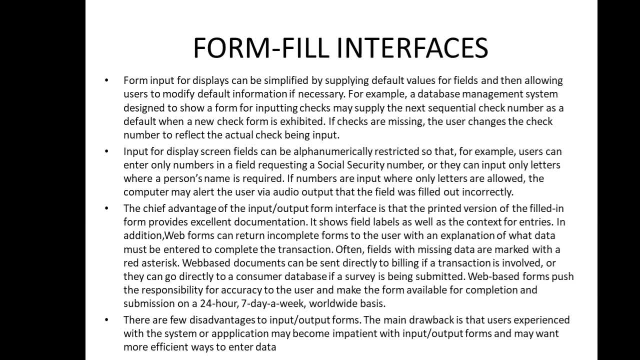 provides excellent documentation. It shows field labels as well as the context for entries. In addition, web forms can form incomplete forms to the user with an explanation of what data must be entered to complete the transaction. Often fields with missing data are marked with a red asterisk. 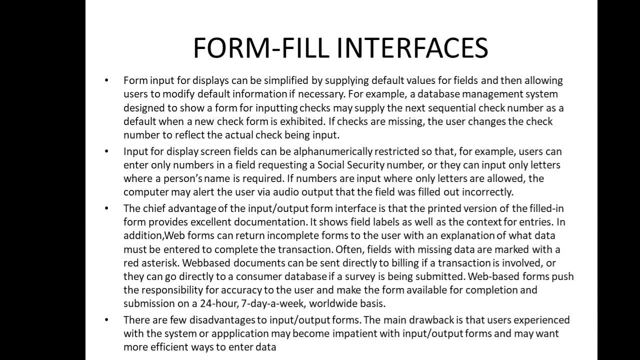 Web-based documents can be sent directly to billing if a transaction is involved, Or they can go directly to a consumer database if a survey is being submitted. Web-based forms push the responsibility for accuracy to the user And make the form available for completion and submission on a 24-hour, 7-days-a-week worldwide basis. 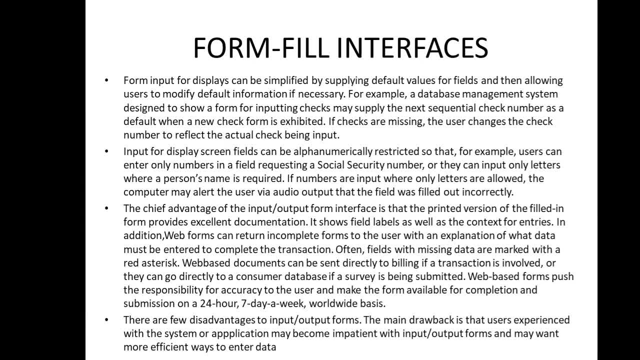 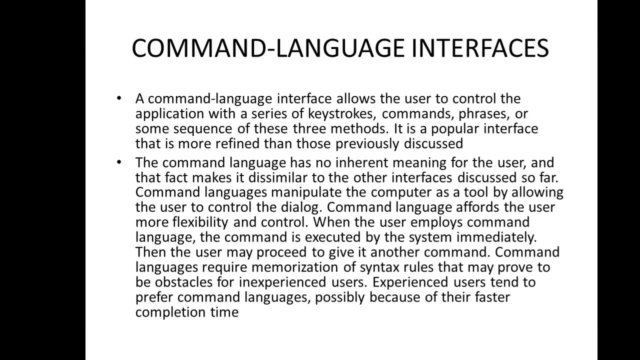 There are a few disadvantages to input-output forms. The main drawback is that the users' experience with the system or application will become impatient with the input-output forms And may want more efficient ways to enter data. Then we also have the command language interfaces. A command language interface allows the user to control the application with a series of keystrokes. 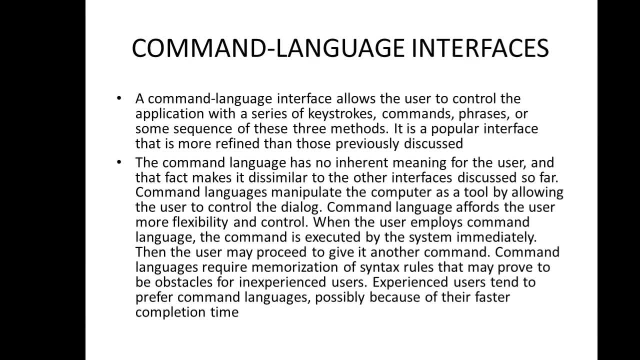 Command phrases or some sequence of these three methods. It is a popular interface that is more refined than those previously discussed. The command language has no inherent meaning for the user, And the fact makes it dissimilar to the other interfaces discussed so far. Command languages manipulate the computer as a tool by allowing the user to control the dialog. 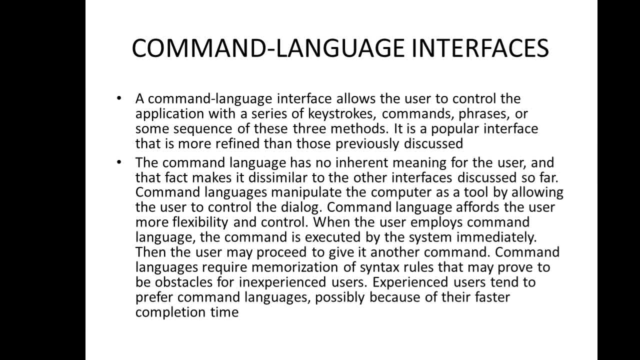 Command language affords the user more flexibility and control. When the user employs command language, the command is executed by the system immediately. then the user may proceed to give it another command. Command languages require memorization of syntax rules that may prove to be obstacles for experienced users. 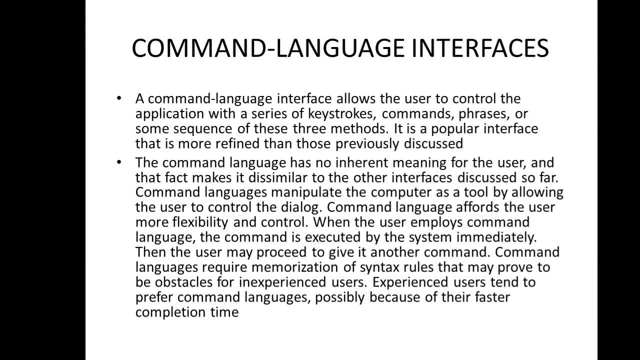 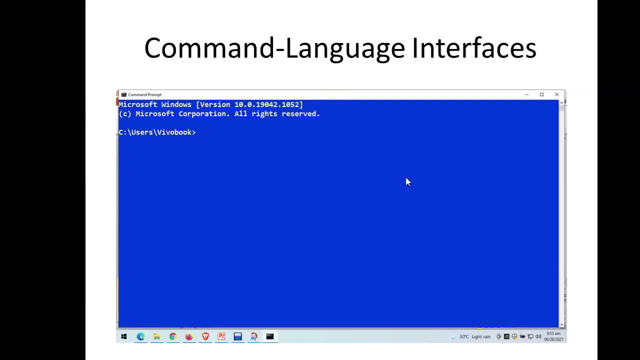 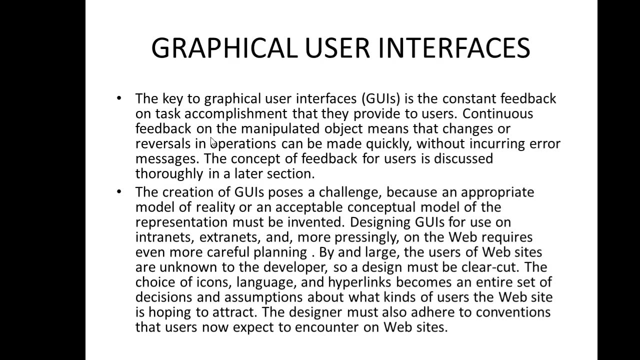 Experienced users tend to prefer command languages, possibly because of their faster completion time. So here's an example of a command language interface to type CMD in Microsoft Windows. Here we can type: here now our command. Now we have the graphical user interface. I know you're familiar with this, So the key 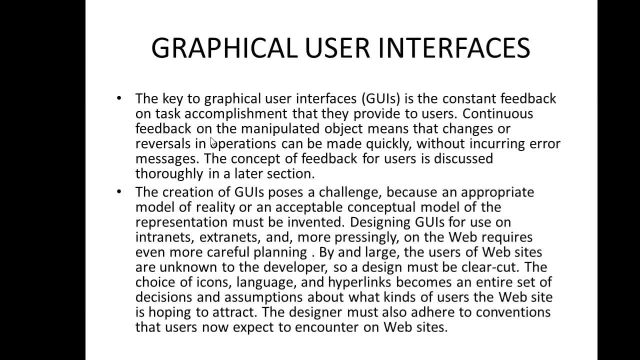 to graphical user interface or GUIs, is the constant feedback on tasks and accomplishments that they provide to users. Continuous feedback on the manipulated object means that changes or reversal in the operations can be made quickly without incurring error messages. The concept of feedback for users is discussed thoroughly in a later section. 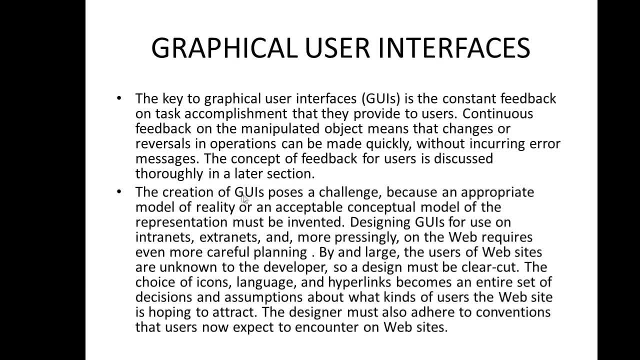 or later video. The creation of GUIs poses a challenge because an appropriate model of reality or an acceptable conceptual model of the representation must be invented. Designing GUIs for use on intranets, extranets and, more pressingly, on the web requires 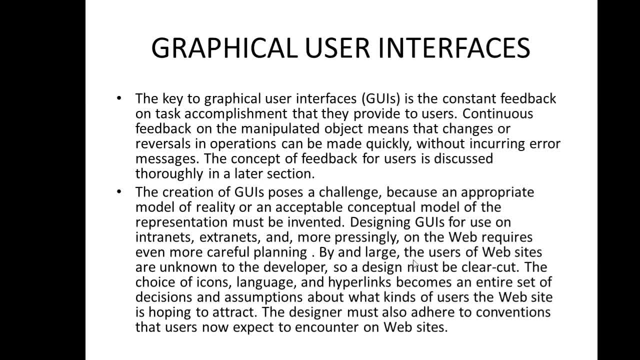 much more careful planning. By and large, the users of websites are unknown to the developer, so a design must be clear-cut. The choice of icons, language and hyperlinks becomes an entire set of decisions and assumptions about what kinds of users the website is hoping to attract. The designer must also adhere to. 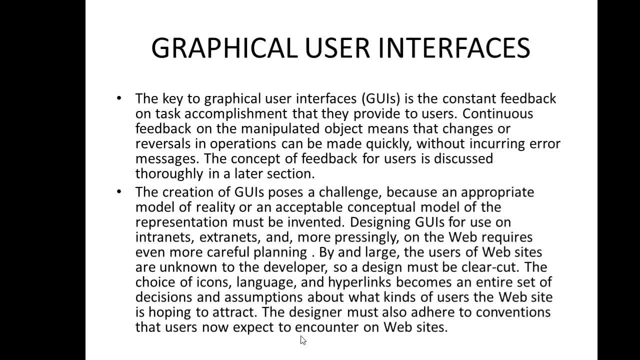 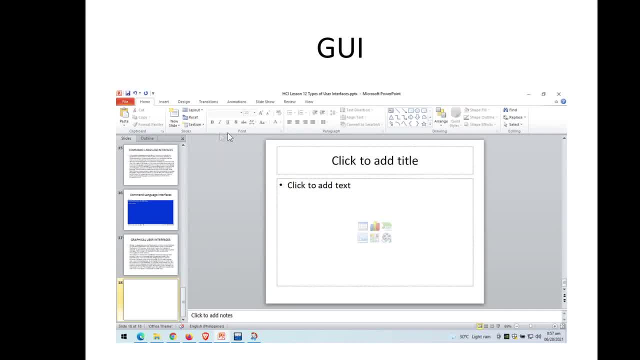 the conventions that users now expect to encounter on the web websites. so here's an example of a graphical user interface. so this is actually PowerPoint. so we have menus, we have icons and we can have also the pointer, etc. and of course, you have the windows. so here's. 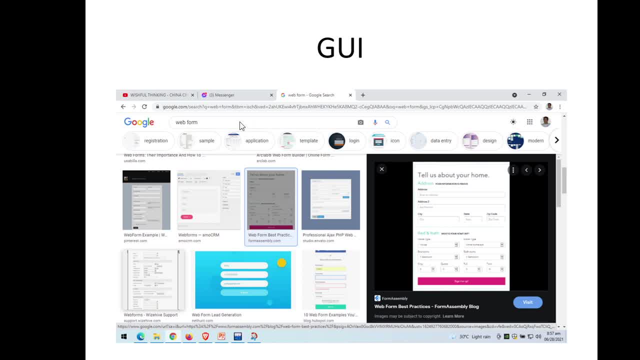 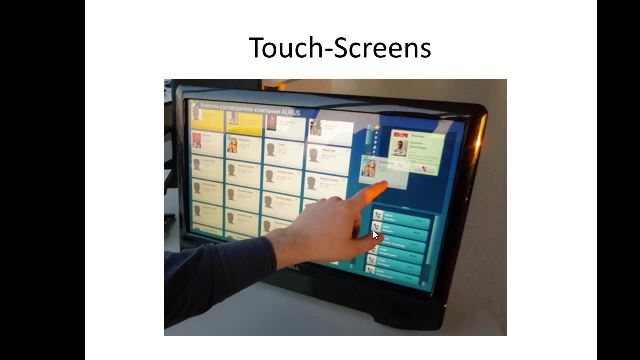 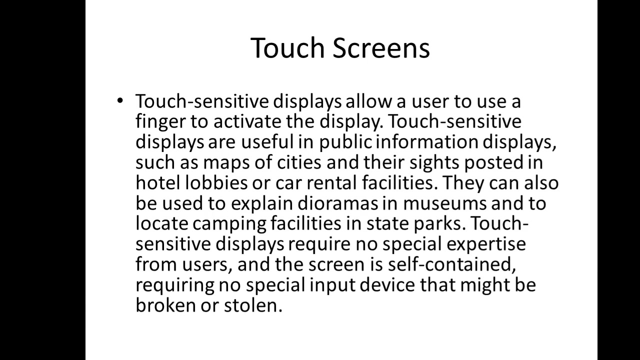 another example: this is a browser, so we have icons. yeah, we have here menus here. then these are now touch screens, so this is our other interfaces. so we have the touch screen user interface. so the text screens or that sensitive displays allows a user to use a finger to activate the display. that's sensitive. 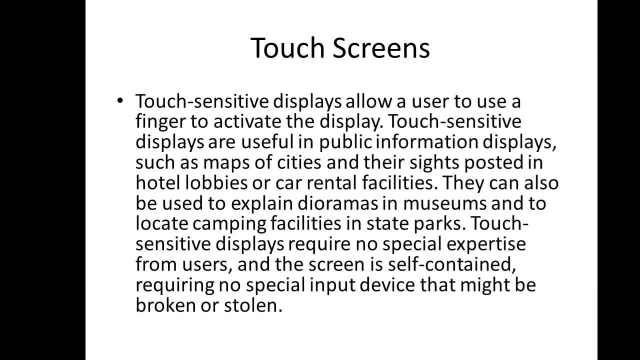 displays are useful in public information displays such as maps of cities and their sites posted in hotel lobbies or car rental facilities. they can also be used to explain dioramas in museums and to locate camping facilities in state parks. touch sensitive displays require no special expertise from users and the screen is self-contained, requiring no. 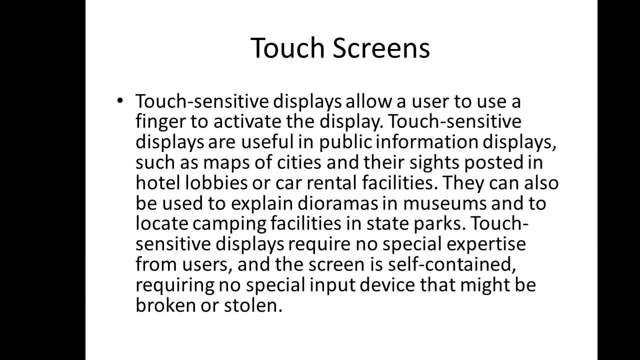 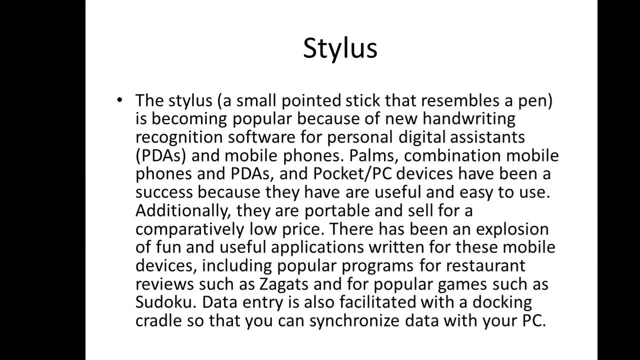 special input device that might be broken or stolen: stylus. the stylus is a small pointed stick that resembles a pen. it's becoming popular because of the new handwriting recognition software for personal digital assistants and mobile phones. palms combination mobile phones and PDAs and packet PCs devices have been a success because they have they have. 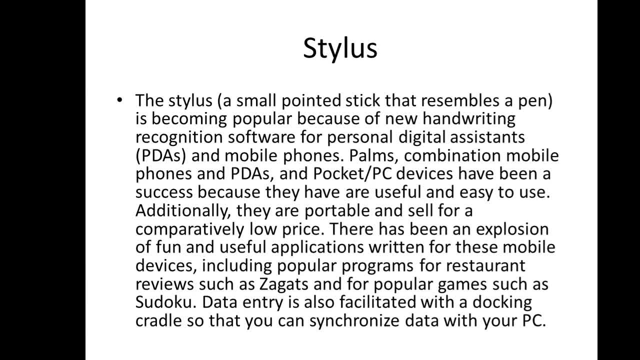 because they have are useful and easy to use, so I don't know how I think there's something wrong. additionally, they are so, but we know that they are useful and easy to use, so, additionally, they are portable and sell for a comparatively low price. there has been an explosion of fun and useful. 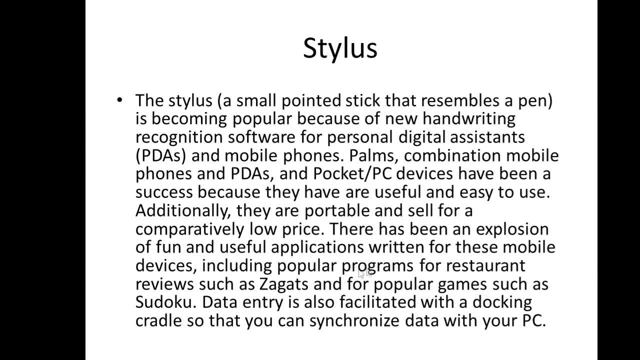 applications written for these mobile devices, including popular programs for restaurant reviews, such as sagas, and for popular games such as sudoku. data entry is also facilitated without communication. so the I am, I was恭喜 with green so that everyone on the top part of me is still a logical breathing. 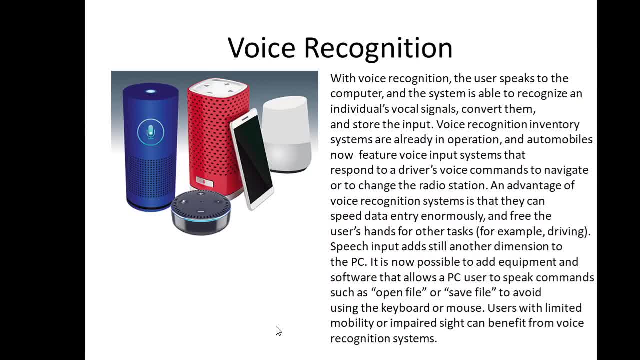 pocket deep into our rupees. so with voice米 recognition the user speaks to the comply ana system. ok with 06. I need to go book books getting those who burn down and store deductible. voice recognition and better examples are already a new achieved. who are the mobiles HR?